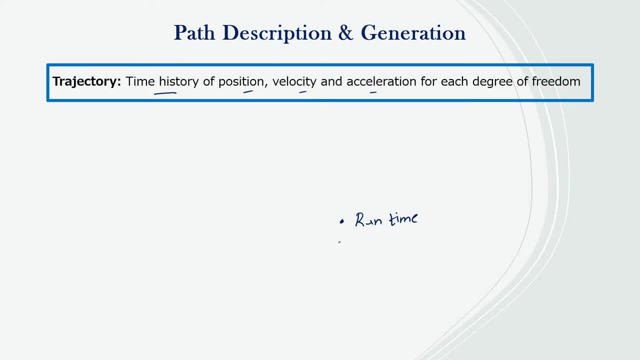 The individual points along a trajectory are computed at a rate called the path update rate, which is, in essence, the rate at which the next point is going to be calculated. This is typically done at a rate of about 60 to 2000 Hz, depending on the robot. 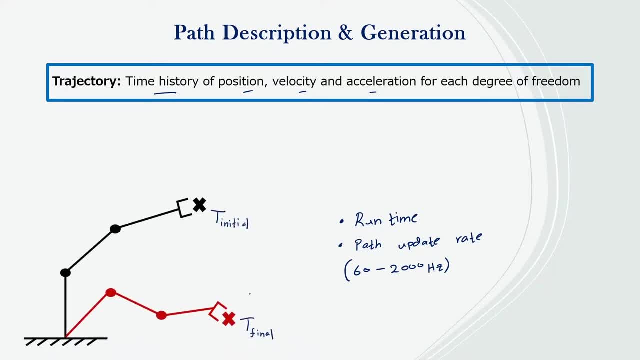 So the robot, as shown here, moves from its initial to its final position. This movement requires a change in both orientation and position of the robot manipulators relative to its base. Now, there are multiple paths that a robot can take. For example, it can follow: 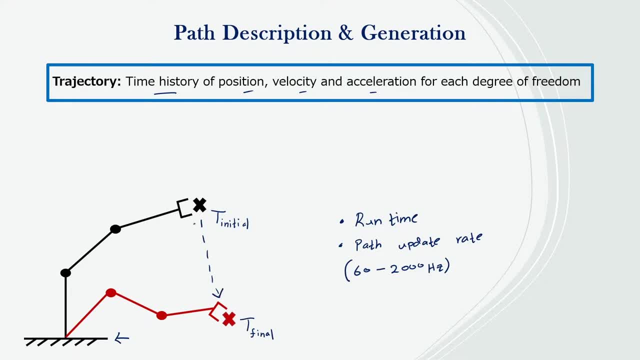 a straight path, or it can even follow a curved path, given no singularities are reached. So, as the user, we let the robot worry about how it should position its joints and links and we only look at the movement of the final frame or the tool frame. Just a note: the 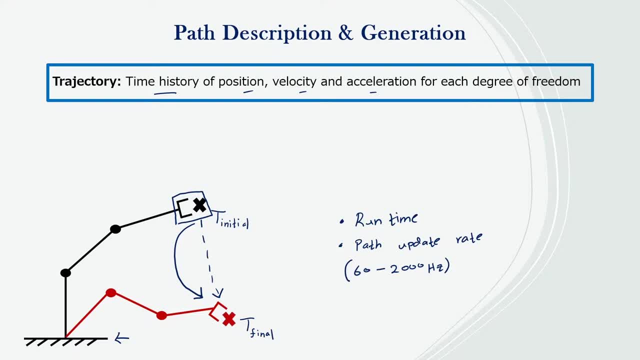 transformation matrices for the robot links can be calculated using inverse or direct kinematics and I have run through some of these matrices in my previous videos, So if you have any questions, please feel free to ask them in the comments section below. And if you have any questions, 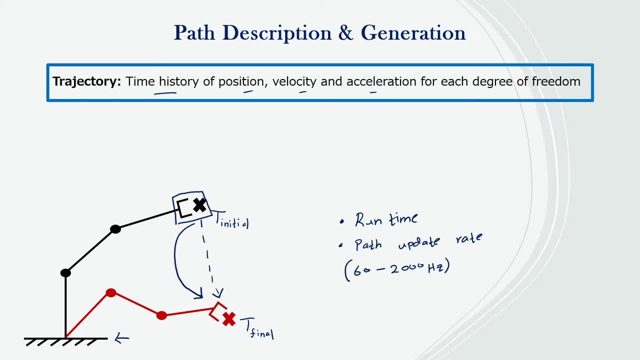 please feel free to ask them in the comments section below. Now, in general, it is preferable to have a smooth motion or a smooth path for the robot, And the reason for this is because if the robot has a sudden movement or a jerky movement, 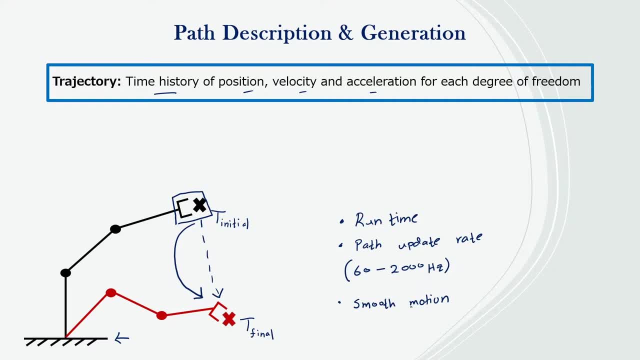 it can lead to vibrations in the robot links. So, in essence, a smooth motion would reduce the wear and tear. Now, as the user, instead of just specifying the initial and final point, we can also specify intermediary or auxiliary points for the robot to move through. So these intermediate points, 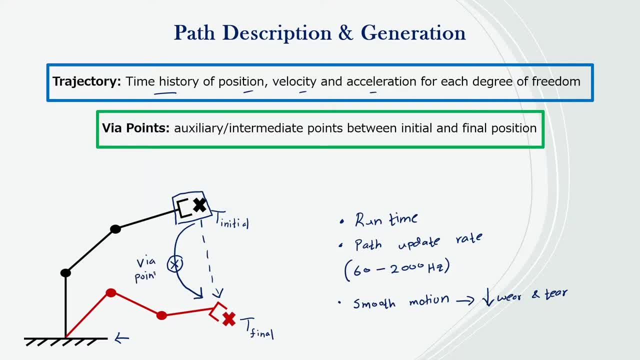 are known as wire points, And the purpose of using wire points is to ensure the robot follows a smooth motion, And this is done by placing constraints on the wire points. So, to ensure the robot follows a smooth motion, we place constraints on the wire points and 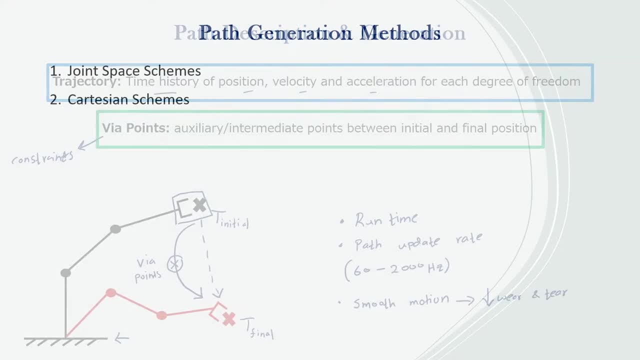 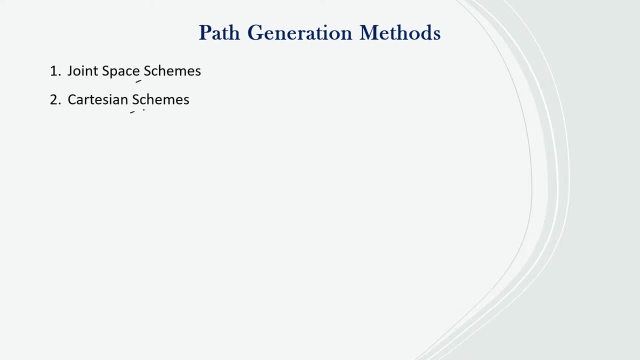 we'll have a look at that in the slides to come. Moving on with regards to path generation, there are two main methodologies, which are joint space and Cartesian methods. With regards to joint space, the planned paths are described using functions of joint angles. 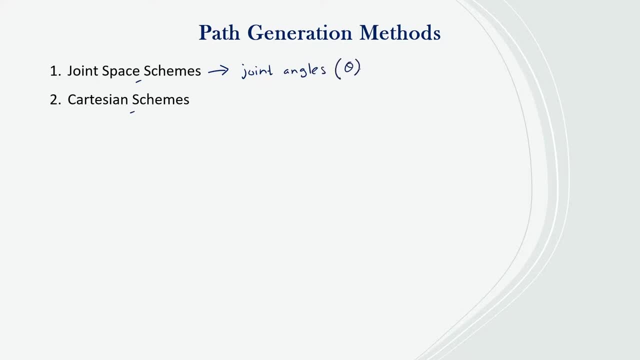 usually in terms of theta. So in this method, each wire point, including the initial and final points, are converted into a set of joint angles using inverse kinematics. On the other hand, the Cartesian scheme directly uses the position and orientation of the robot frames, along with the path points as specified. 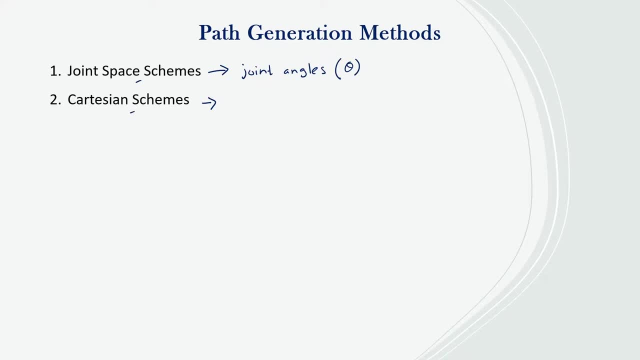 by the user to generate the trajectory. In general, joint space schemes are easier to use and compute. This is mainly because Cartesian schemes require inverse kinematics to be used to calculate the position and orientation at every single point along the path, as per the path update. 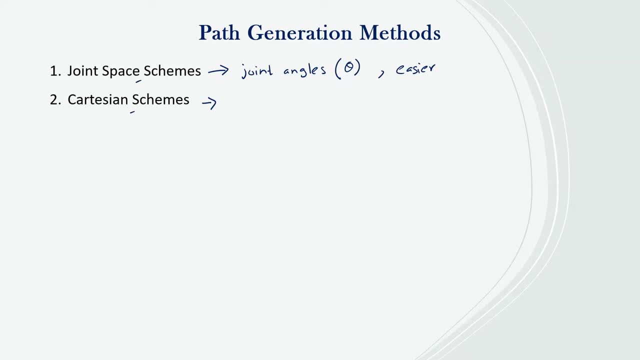 rate, So they have a higher computational burden on the robot. In this video we will only look at joint space schemes Now. this can be split into two sub-methods, the first being cubic polynomials and even higher order polynomials. however, 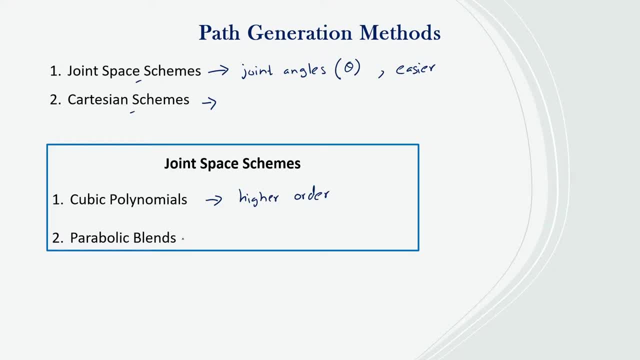 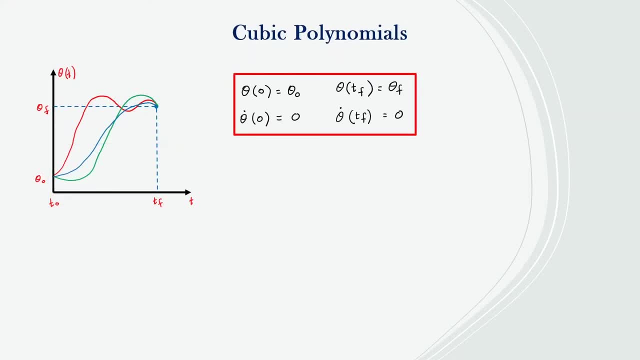 I won't look at that here, The second being parabolic blends. So let's get into that Right. so now we will look at cubic polynomials. As you can see, here there are multiple paths that can be taken for the robot to move from. 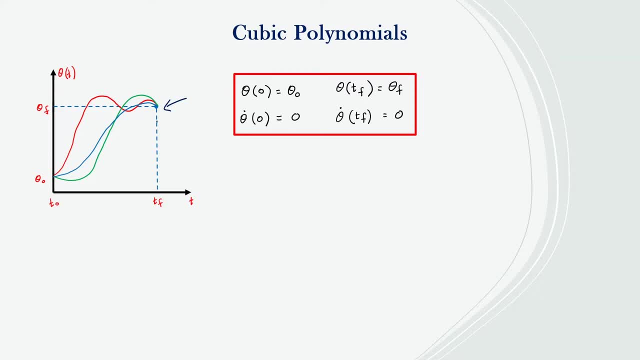 its initial to final position. So what we would really want is a set of functions or a function that can describe each joint where, at time t0,, the initial position is theta0, and at time t0,, the initial position is theta0, and at time t0,, the initial position is theta0, and at time t0,, the initial position. 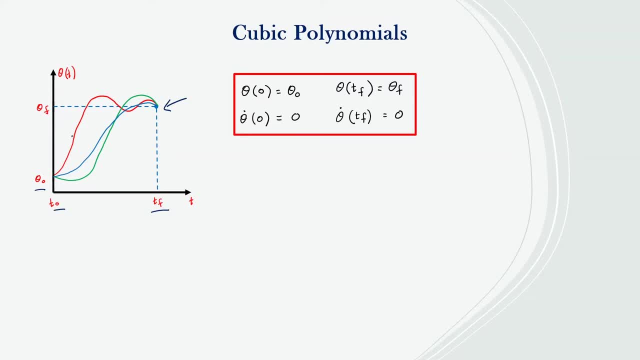 is theta0.. Now let's look at the final position at time tf, the final time. the final position is at theta f. Now, like I mentioned earlier, it is important for the robot to follow a smooth path and to ensure that happens, constraints are placed. 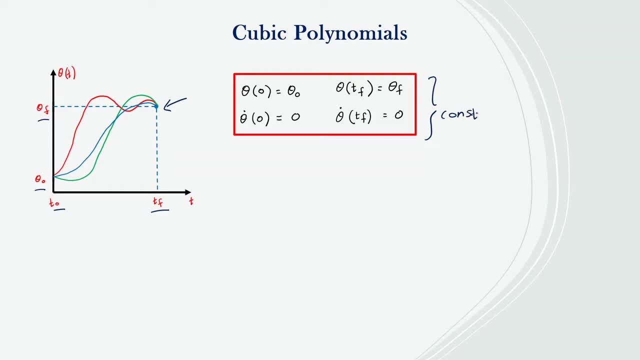 So these are the constraints that we will look at Right. so there are four constraints. The first two are that at the initial position, at time 0, the angle should be theta0, and at the final position, at time tf, the angle. 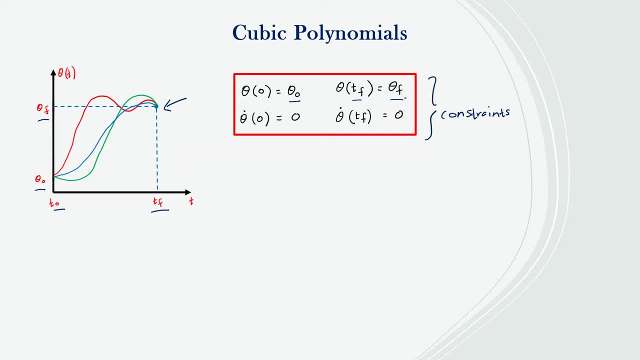 should be thetaf. it is also required that this function be continuous in velocity, hence the initial and final velocities are both 0. now, these four constraints can only be satisfied by at least a third order equation, hence cubic polynomials. so this equation would take the form of this: where you have a 0 plus a 1 t plus a 2 t. 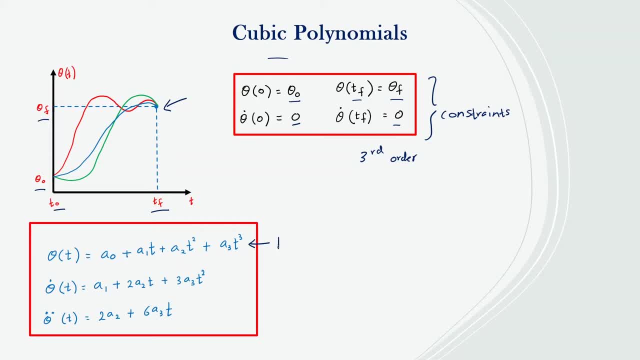 squared plus a 3 t cube, and this equation will represent the position. its derivative, theta dot, would represent the velocity and its double derivative, theta double dot, represent the acceleration. so what we want is a function that represents the trajectory, and this function is this equation for position. 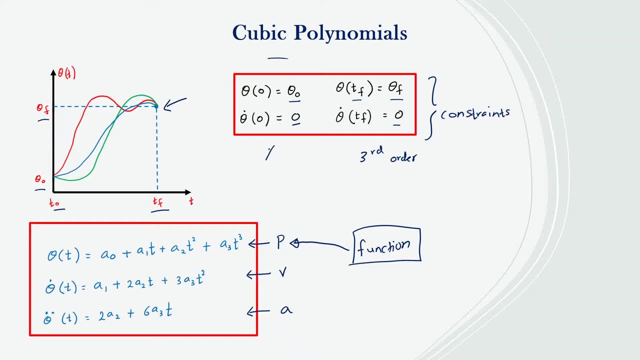 right here. so what we would need to do is use the constraints to find, along with these equations, to find the coefficient of velocity and the coefficients a0 to a3, and thereby come up with an equation that represents the trajectory that the joint or the manipulator should take, so to make. 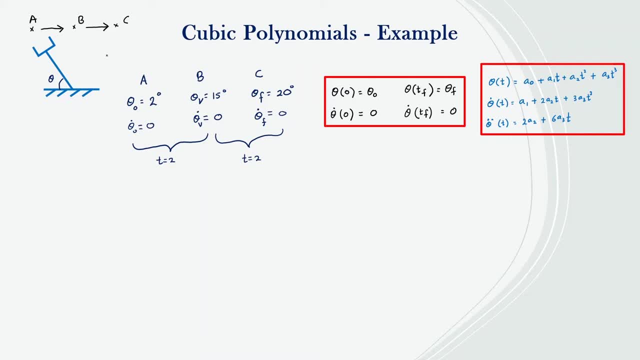 things clearer. let's go through a worked example. this question is for a 1 degree of freedom robot manipulator. as shown here, it moves from point A to point B and then to point C, so point B is actually a via point. it starts off at 2. 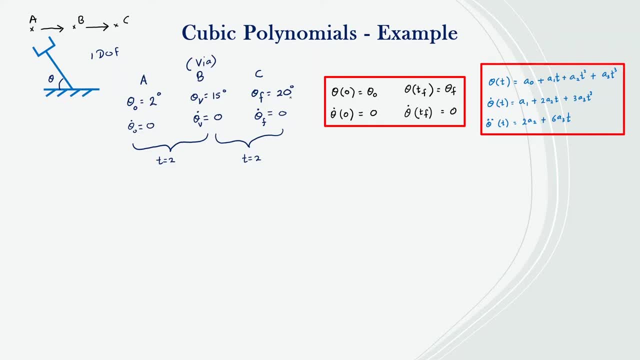 degrees, then 15 degrees and finally 20 degrees. the initial and final velocities are both 0, which satisfy the constraints as shown over here. the time from A to B is 2 seconds and another 2 seconds from B to C. something you should note here is the velocity at point B and 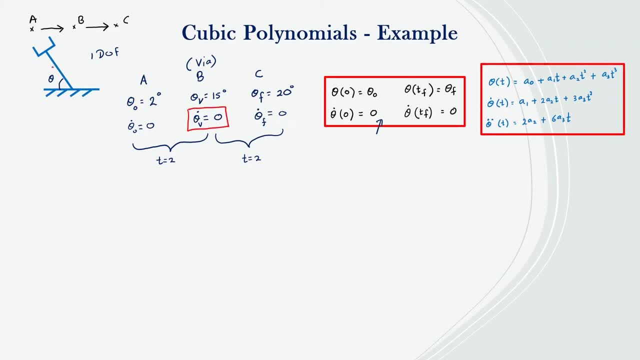 I have set that to be 0, which means the robot moves to point B and comes to a momentous rest before moving from B to C. now for a practical robot, or applying this scenario practically. you wouldn't want the robot to stop at point B, you would want a continuous motion from A to 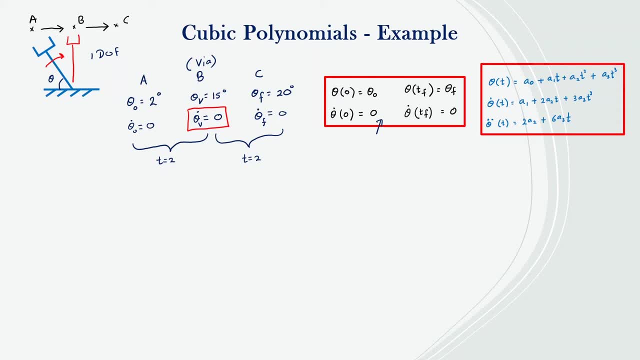 B and B to C. you would not want the robot to come rest at point B, but I have done this for the simplicity of this question, so that we can simply understand how to apply these equations and constraints to solve cubic polynomials. so our final outcome would be two functions or two equations: one: 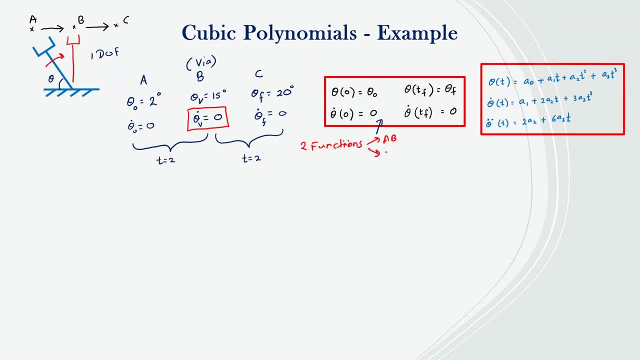 for the motion from point A to B and another one for the motion from point B to C. for both these equations we will apply it from time T equals 0 to 2 seconds, and the same for the second equation as well. so let's see how we can do this right. so we will start off for 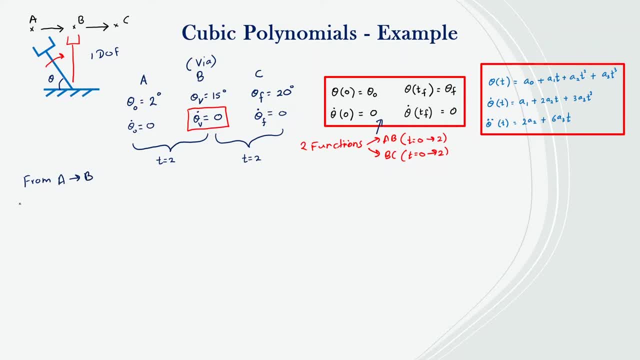 the motion from A to B. at 0 time time T equals 0, so we can use our very first constraint. we know theta 0 is equal to theta naught and theta 0 is equal to this equation. here at time T equals 0, so we can put that in: a naught plus a 1, 0 plus. 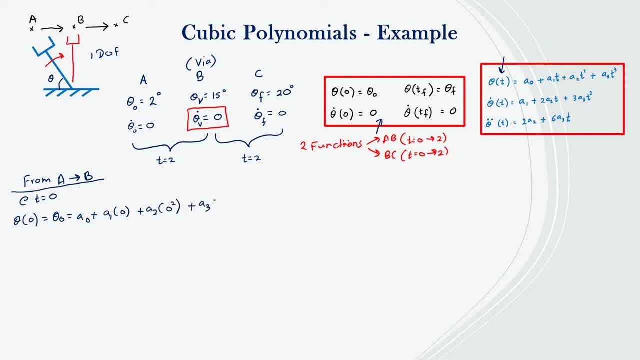 a 2, 0 squared plus a 3, 0 cube, theta naught is equal to 2 degrees, and if you solve this equation, you would get a naught equals 2, which is the first coefficient to found. we can then look at the second. 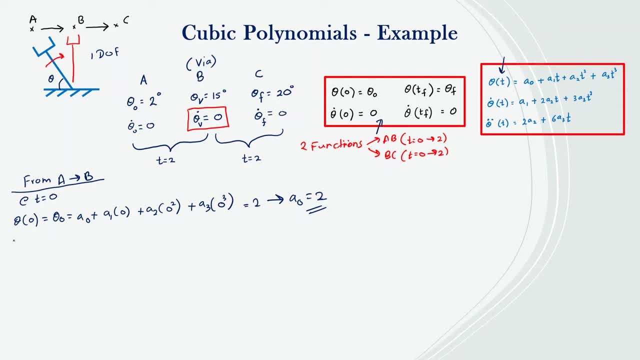 constraint: theta dot 0 equals 0 and theta dot 0 is equal to this equation over here, which is a 1 plus a 2, T 0 plus a 3- sorry, it's 2a 2 and 3a 3: 0 squared. 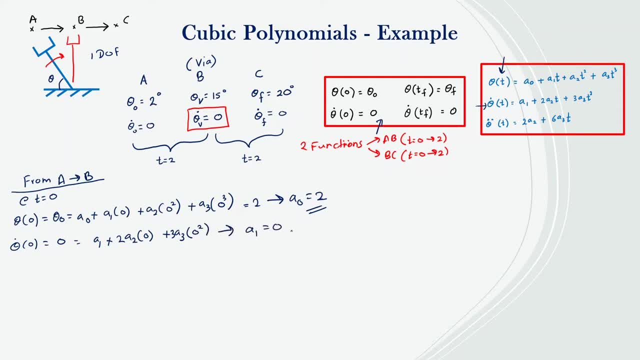 And if you solve that equation, you would get a 1 to be equal to 0, which is the second coefficient. Now we can look at the scenario: at time, t equals 2 seconds, So at this point the robot is at point B. We can apply these two constraints again, but this time in terms of TF, because we're considering a to B as one motion. 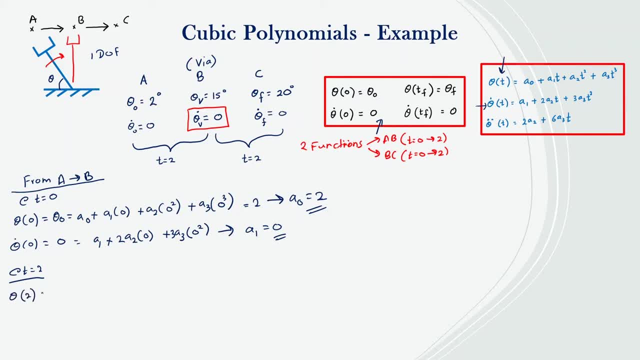 so theta at 2 would be equal to a naught. We know the value of a naught: It's 2. a 1 t. We know a 1 is 0, so we can omit that term. We can straight away move on to a 2 t squared. t is 2, so 2 squared. 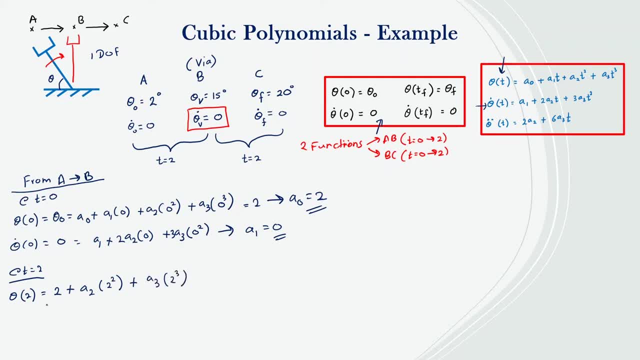 plus a 3, 2 cube. We know at time t equals 2, the angle is theta V, which is 15 degrees, So that's equal to 15. Rearranging this equation should give you 4 a 2 Plus 8 a 3 is equal to. 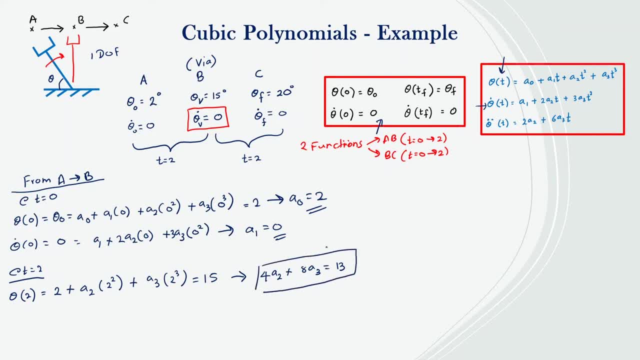 13. So that is the first equation. The second equation can be found by looking at the velocity. theta dot at 2 is equal to 0, Which is equal to a 1. we know a 1 is 0. will omit that term. 2 a 2. 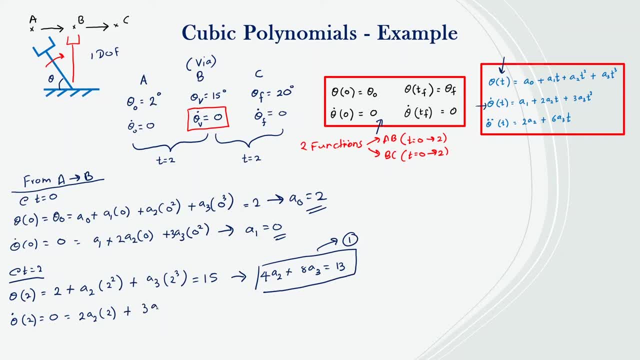 t is 2 plus 3 a 3, 2 squared, and Rearranging this equation should give you 4 a 2 Plus 12 a 3 is equal to 0, And this is the second equation Right, so 1 and 2 can be solved simultaneously. 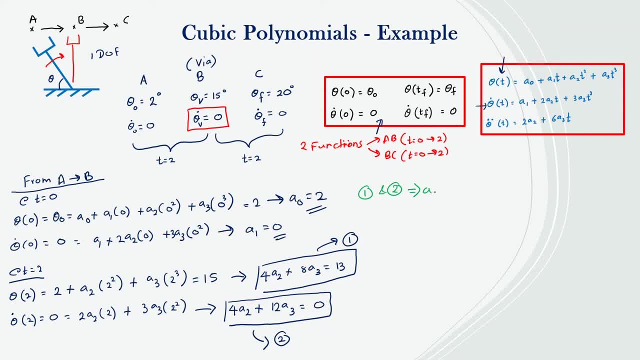 and if you do so, you should get a 2 to be equal to nine point seven, five, and A 3 as being equal to negative three point two, five. So you found the coefficients. all four coefficients is 0 to a 3 for the first motion, a to B. you can repeat these steps. 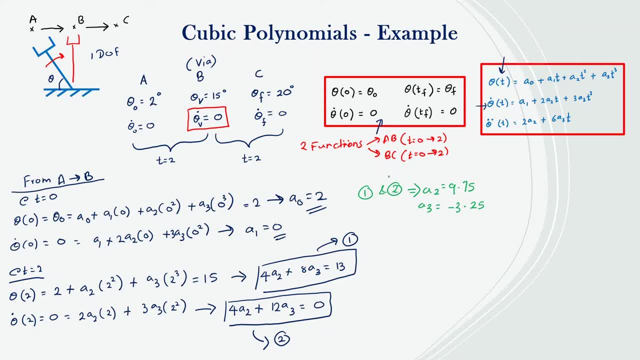 For B to C and you will find the next set of coefficients, considering at time t equals 0 when the robot is At B, and at time t equals 2 when the robot is at C. and if you do that, You should get these as your four coefficients, from B 0 to B 3. 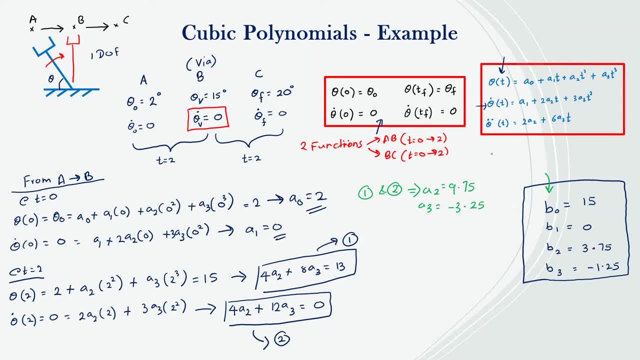 The final step will be to put these coefficients back into this equation here Proposition, and it would give you an equation or a function For the trajectory from point A to B and then from point B to C, and you should get this as your final answer When you put your coefficients back into the original equation. 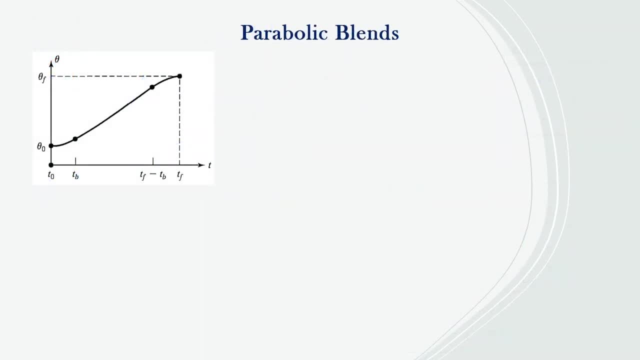 Right. so now we move on to parabolic blins, which is another method in the joint space schemes: a cubic polynomial. A cubic polynomial would follow a curved path, But a linear or a straight path could also be followed. It should be noted that even if the joints of a robot follow a relatively straight path, 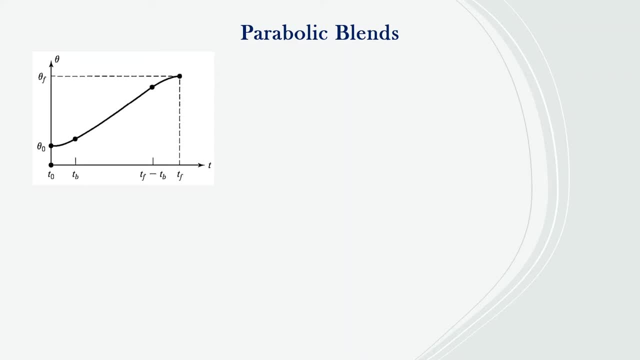 The final frame or the tool frame may not necessarily follow a straight path. There is, however, a problem with a linear or straight path Or straight path, and that is discontinuous velocity At the beginning and end. This problem can be solved using parabolic blends in these regions over here. 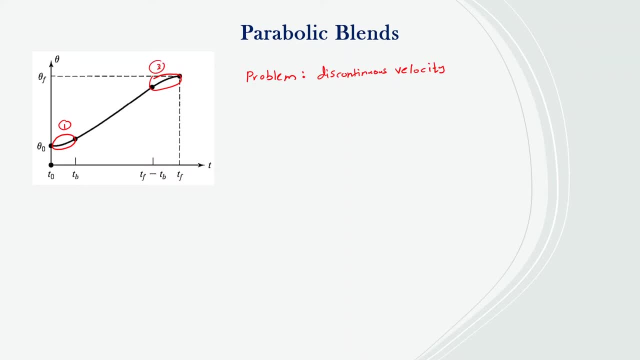 So this is the first blend. This is the second parabolic blend. at the beginning and the end and in the middle We have the linear region. So the blends ensure that there is constant acceleration. So The constant acceleration ensures a smooth change in velocity from the blend to the linear region and vice-versa. 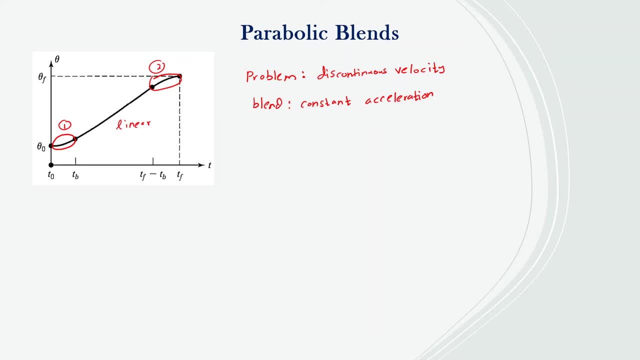 This in turn ensures that the position and velocity are continuous. So the constraints, as described previously, are satisfied. Now there are three variables that have to be looked at when solving parabolic blends, and those are: theta B, which is the joint angle at the end of the blend region. 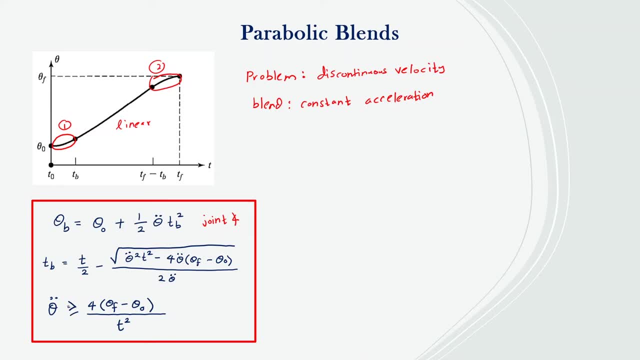 Tb, which is the blend time or the blend duration, and theta double dot, which is the acceleration. So it is normally assumed that theta TB- Sorry TB- for blend 1, Which is the duration for blend 1, is equivalent to the duration for blend 2. 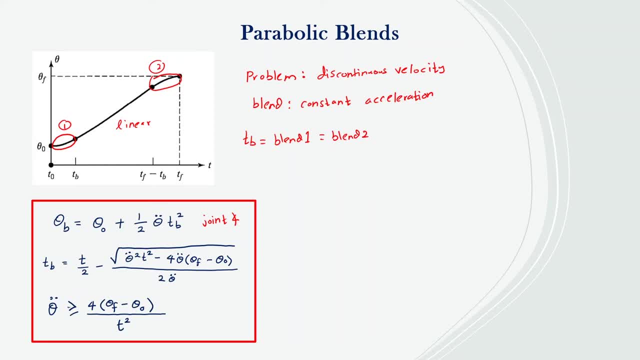 Now, using these three variables And the plot as shown over here, Three functions can be calculated or can be derived for the path trajectory Right. so the first function, which exists from time 0 to TB, describes blend 1. the second function, which is in this region, TB to TF minus TB, describes the linear region. and 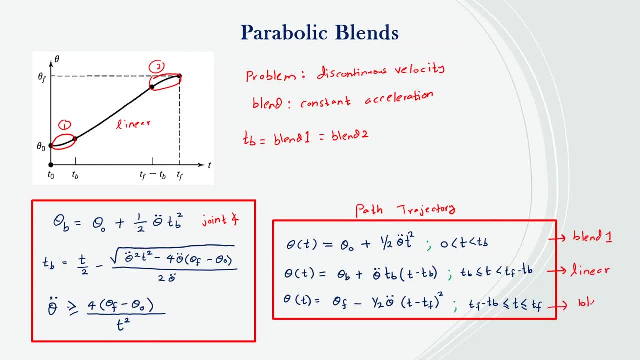 The third function is for blend 2, from TF minus TB to the final time TF. so our final outcome would be to solve and Provide these three functions which describe the path trajectory For the parabolic blends which involve the blend first blend region, linear region and the second blend region. 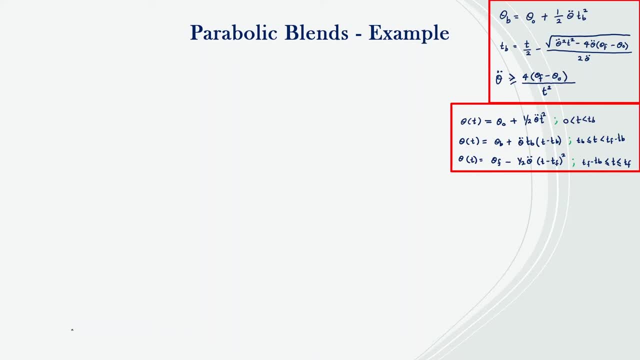 Right. so to make things clearer, let's go through a work example for parabolic blends. The question is quite simple. We move from point A to point B, our initial angle is 15 degrees, theta naught and theta F is 75 degrees. Both initial and final velocities are 0 and the duration for the motion is 3 seconds. 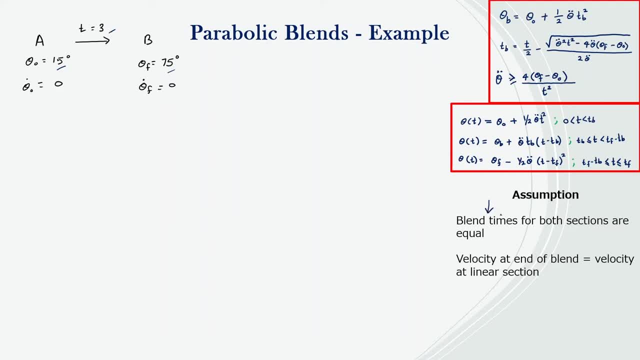 We assume that the blend times for both blend regions, 1 and 2, are equal and that the velocity at the end of the blend Region equals the velocity at the start of the linear section, due to the constant acceleration. So we can start off by calculating theta double dot, which is the acceleration. 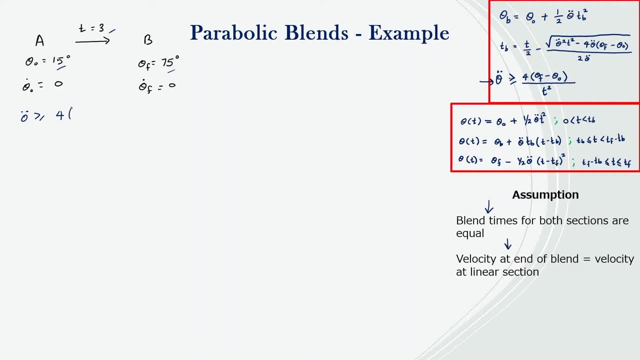 So theta double dot is greater than or equal to 4 times theta F minus theta naught, Which is 75 minus 15, divided by T squared, which is 3 squared, This has a numerical value of 26.7 degrees per second squared. So usually we don't use this value, but we would prefer to choose a value slightly greater than this. 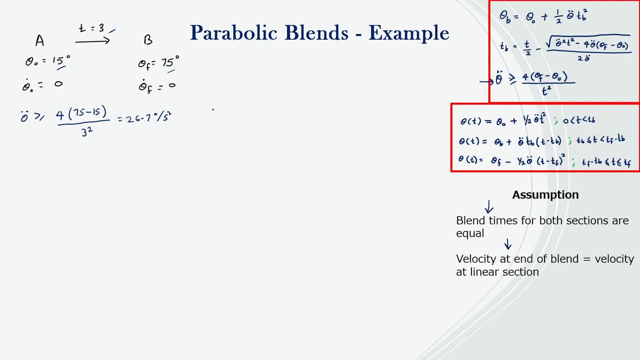 You're free to choose any value Greater than 26.7. but for the simplicity and ease of this question, I'm going to choose theta double dot as being equal to 30 degrees per second squared Right. so in a similar manner, Tb and then theta B can also be calculated. and if you do that, 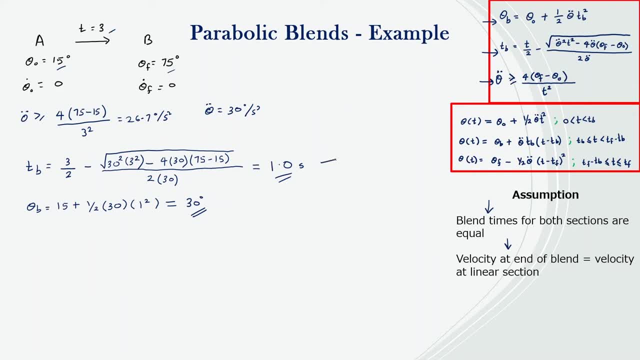 You should get these as your final answers: TBS being 1 second and theta B as being equal to 30 degrees. you can then substitute all these values into these three functions to find the path trajectory. so let's have a look at that right. so the path trajectory for. 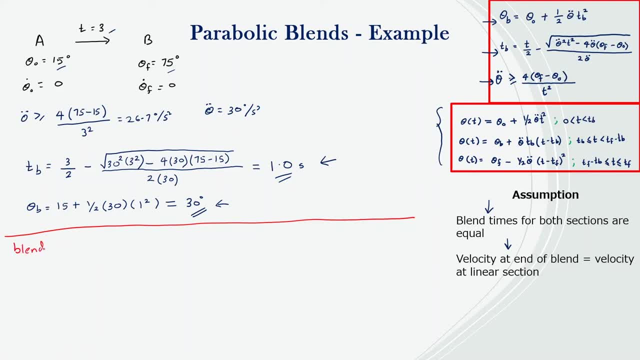 the first blender region is theta T, and that's for the first equation over here, which is from sorry, which is equal to theta naught, which is 15 plus half theta double dot, which is half of 30, again 15 T squared. and this exists for T from 0. 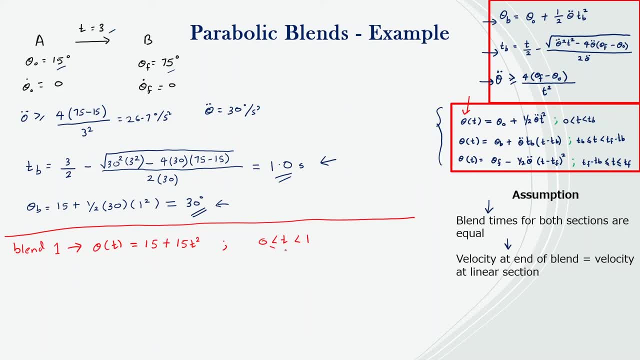 to TB, which is 1 second. the second is for the linear region. theta T is equal to. so now we are looking at the second equation over here. you theta B. theta B is 30 degrees plus theta B- sorry, theta double dot into TB. so theta double dot is 30 degrees into TB is 1 second. so that's 30 times T minus. 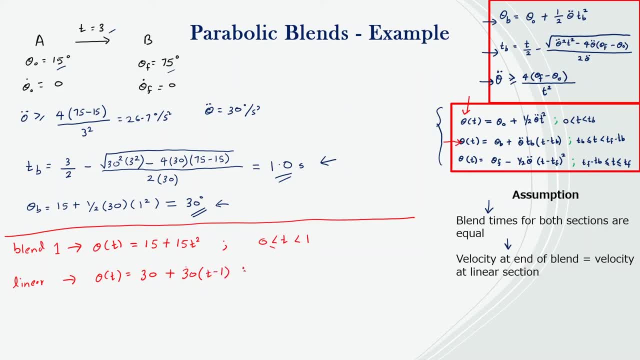 TB, which is T minus 1, and this exists for a time from T which is equal to greater than or equal to 1, less than or equal to 2 seconds. TF minus TB is equal to 2 seconds right, and the final function for the second blend region is theta. T is equal. 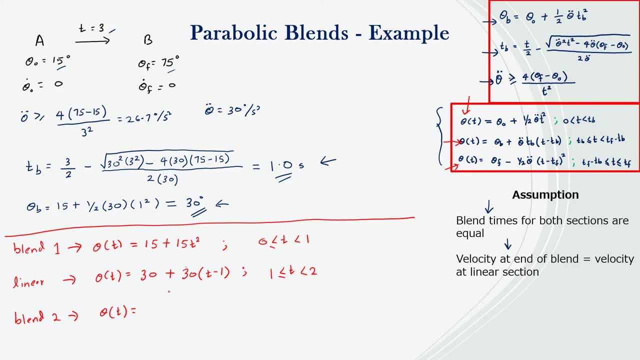 to. and now we are applying the final equation over here: theta F is 75 minus half theta double dot. theta double dot is 30, so half of that is 15 times T minus T F, which is T minus 3. the final time is 3 and that's squared. and this: 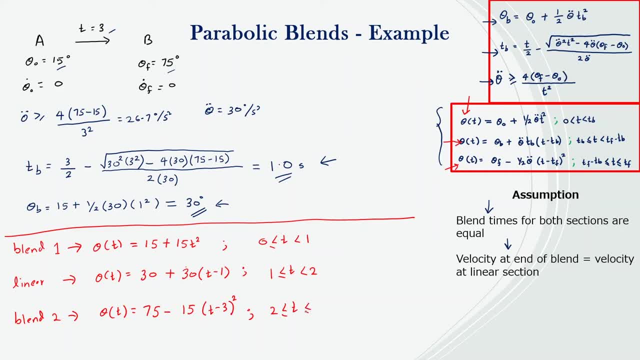 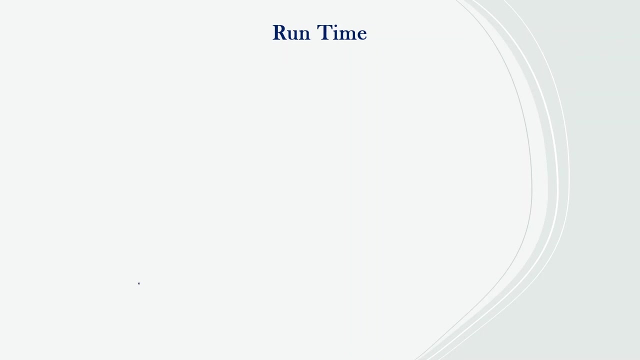 exists for a time from 2 seconds to 3 seconds. so these three functions are final answer and they described the path trajectory. all right, right, so that brings us to an end for this video, but before I finish it off, I would like to briefly talk about what happens at runtime. So a runtime reference is a data, word or animation, we call it a parameter and it Sal company. and simply because of this,